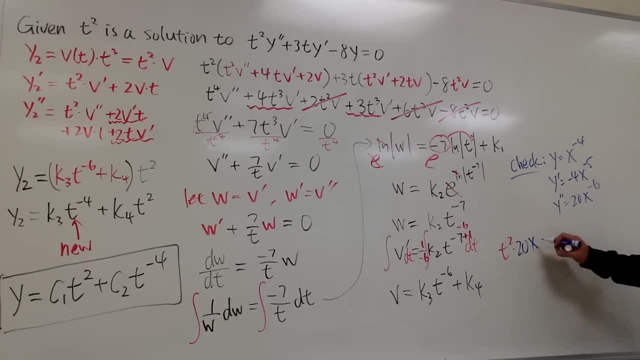 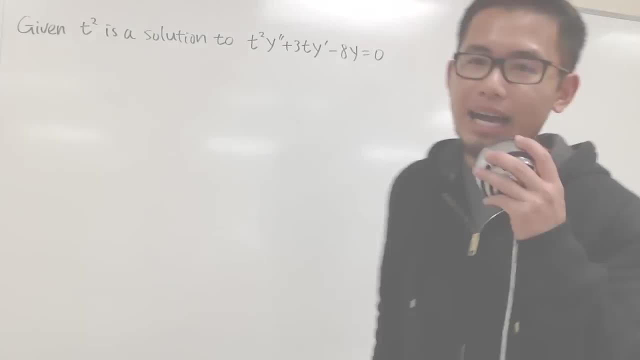 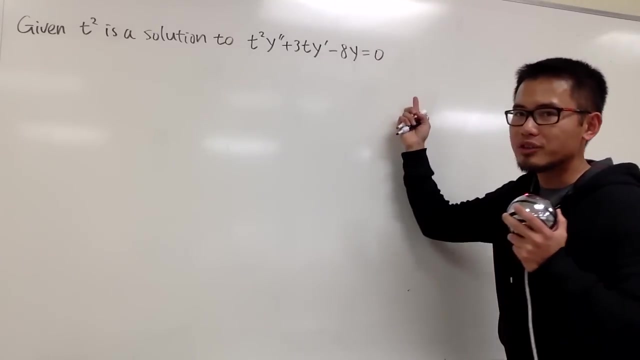 So we multiply by 20x to the. well, I use x. I don't know why I use x. I should use t. I'm going to show you, guys, how to use the reduction of orders to solve this. We are first given that t, squared, is a solution to this differential equation. 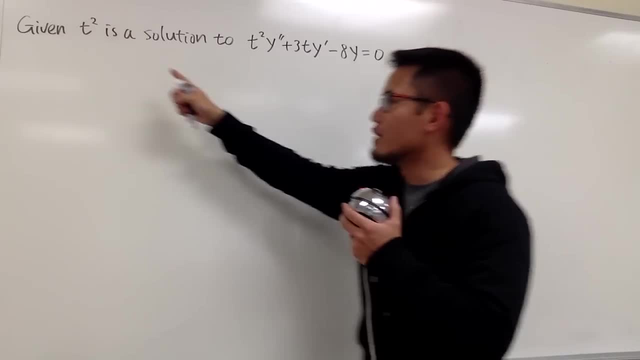 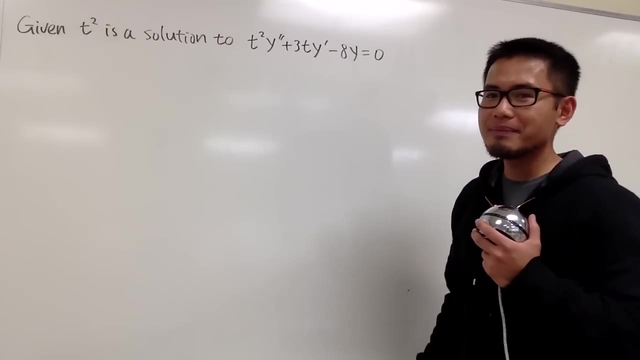 and you should just take a minute or so to verify it yourself. Just derive this twice, plug in and you will see 0 is equal to 0. So it is in fact a solution. okay, And notice that we have a second order because of the second derivative here. 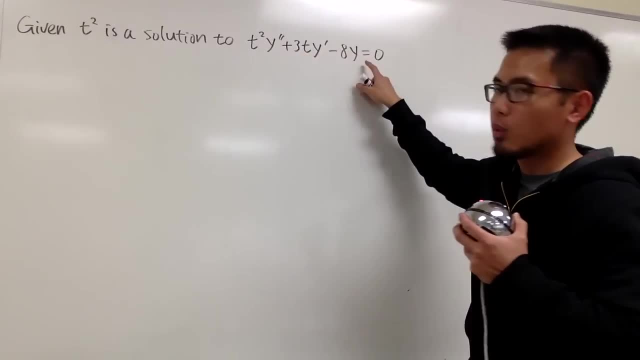 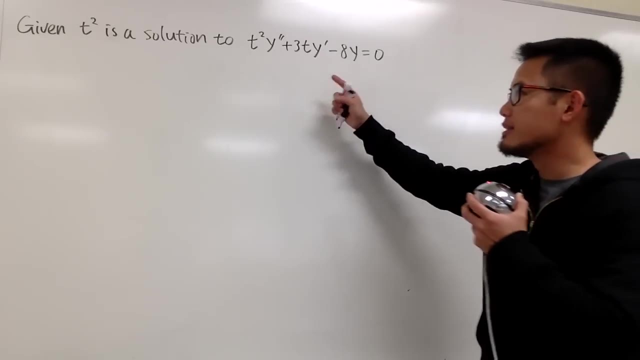 and this is linear, because y double prime and y prime and y, they are all to the first power, right. But in this case the coefficients, they are not constants, because you already see we have a t squared and a 3t here, right. 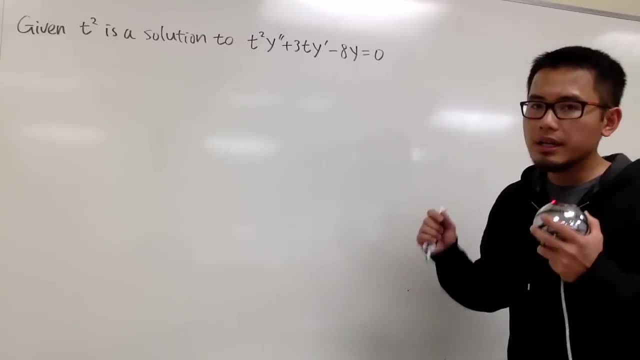 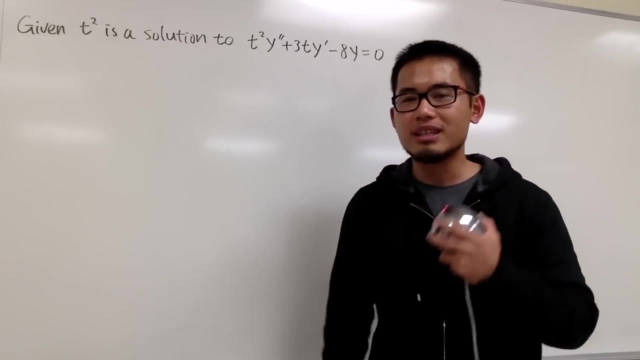 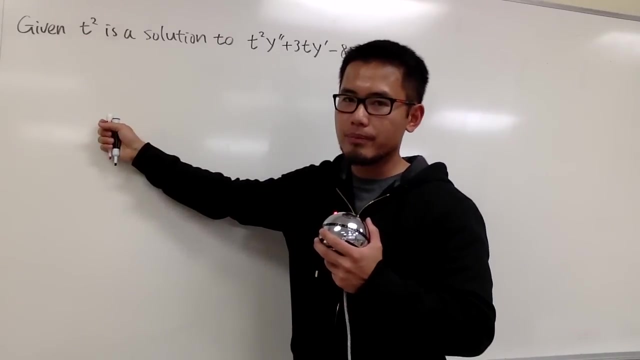 So in our case here we have a second order linear differential equation with variable coefficients. Therefore, we cannot just do the things I told you guys in the previous in this video, namely I cannot just tell you guys that, hey, this is the first building block for the solution t squared. 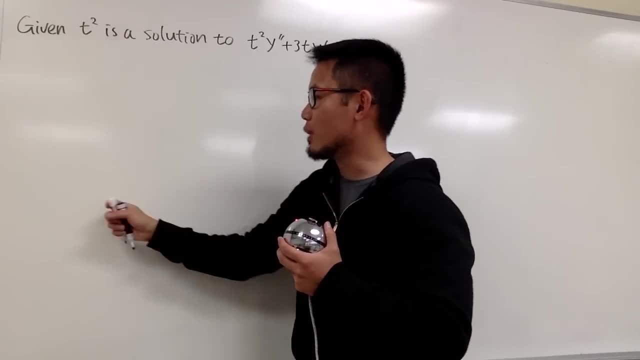 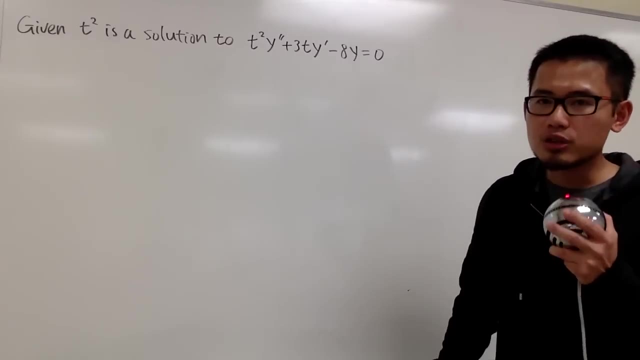 For the second block. can I just do t times the first one, t squared, and say that's t cubed. No, cannot do that. In this case. we really have to use the reduction of orders to figure out what the second building block for the solution would be alright. 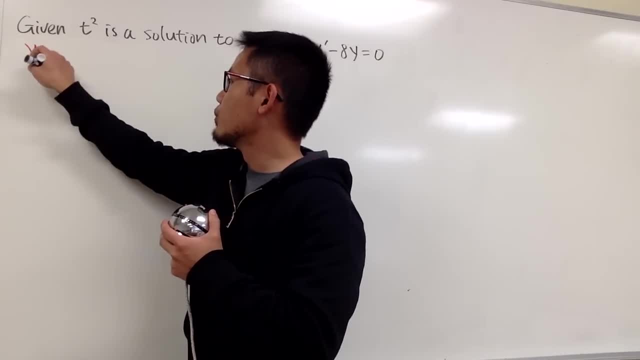 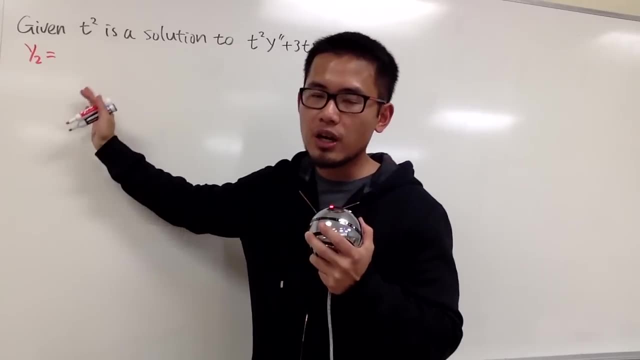 So here we go. Let me just write down y2 right here, and the deal is that first we are not going to solve this, We are not going to worry about the constant multiple yet We are just trying to figure out the building block for the solution. alright, 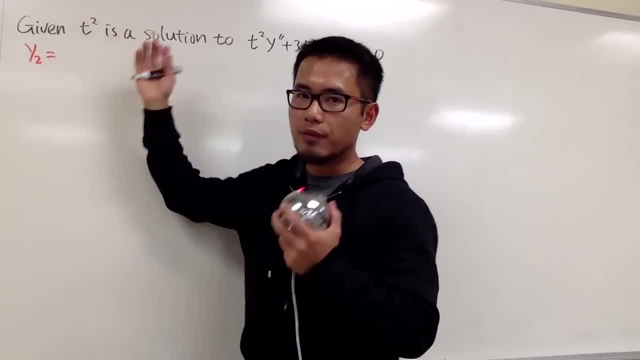 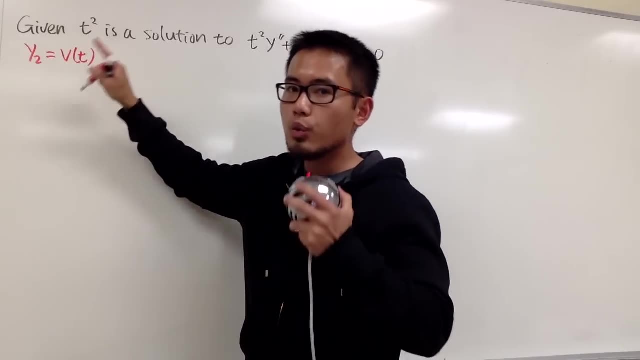 And for y2, since you are given t squared as the first solution right here, y2 will just be phi of t, a function in terms of t. We multiply this right here by the first one, So we multiply by t squared like that: 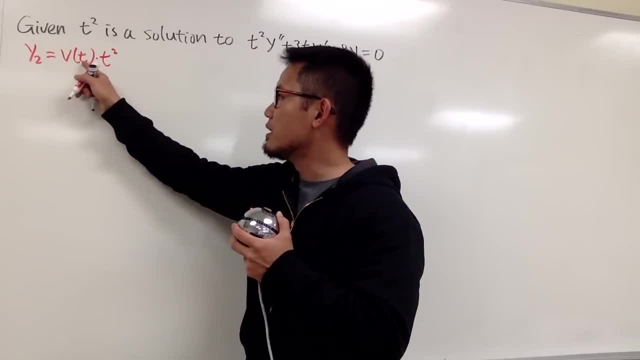 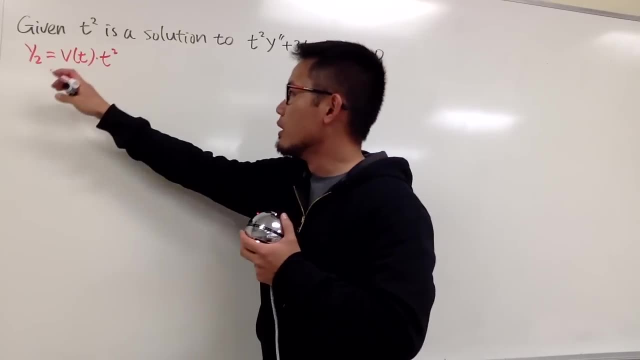 This is the starting. So we put down phi of t times t squared, and then we begin from there, So we can write this equation twice and things like that. Alright, before we differentiate this equation, let me just put this down in a nicer form. 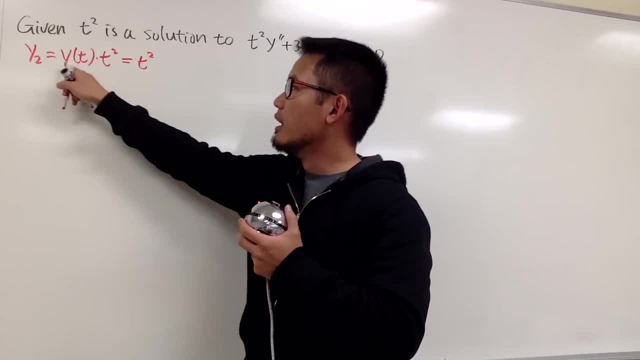 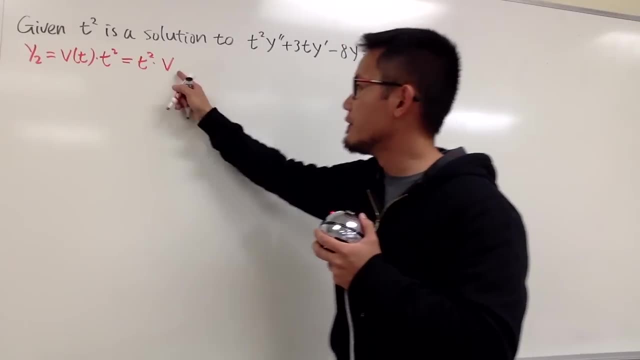 Let me write down t squared first, and then let me just write down, instead of phi of t, just the phi right here. okay, But we have to remember phi is a function of t, Alright, so now let's go ahead and differentiate. 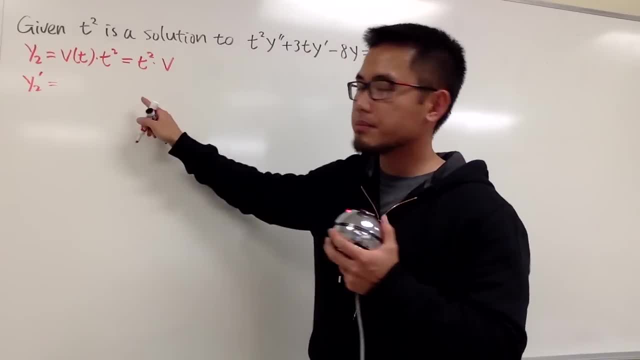 y2 prime. it's going to be here. we have to use the product rule, right? So let me just keep the first function, which is t squared, and multiply by the second, which is t squared, Which is phi prime. 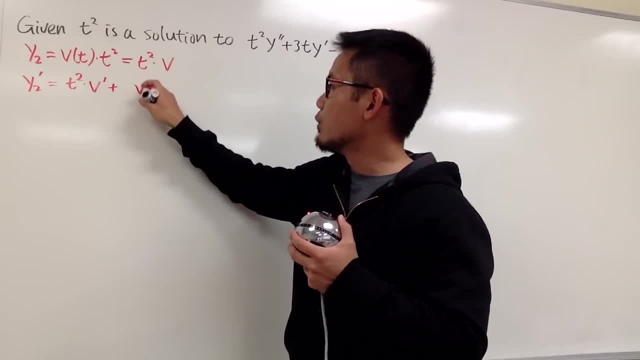 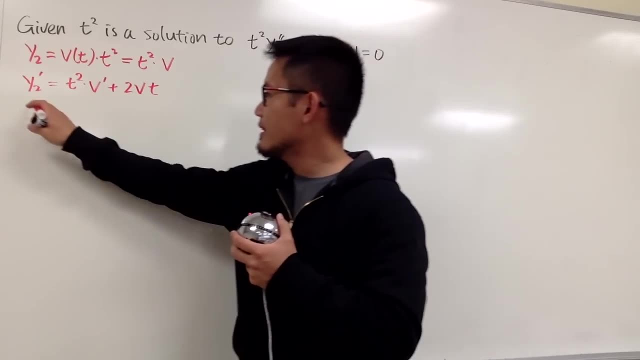 and then we add it with the second function, we keep it and we multiply by the derivative first, which is 2t. so let me put down 2 right here and t right here, like that, And the next derivative by 2 double prime is going to be: 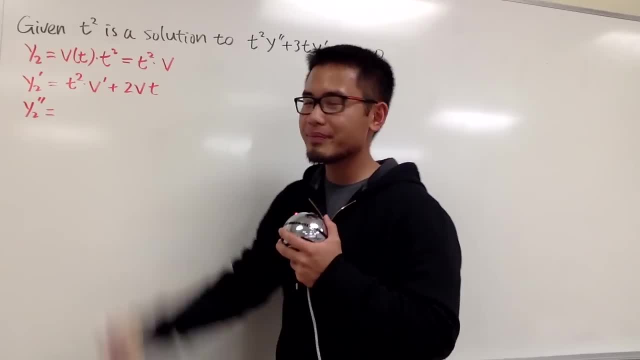 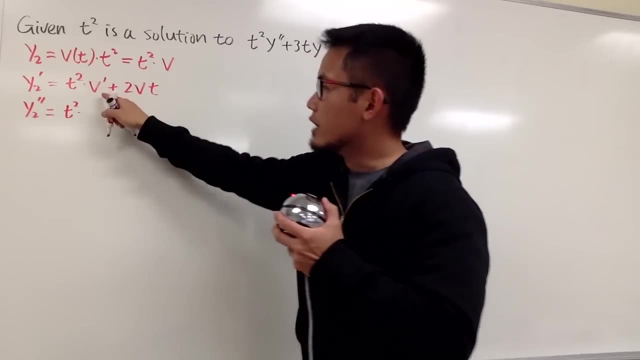 remember to do: product rule here and product rule here. Alright, for this one we keep the t squared first and we multiply by the derivative second Derivative of the first derivative will just be the second derivative right. So we have phi double prime. 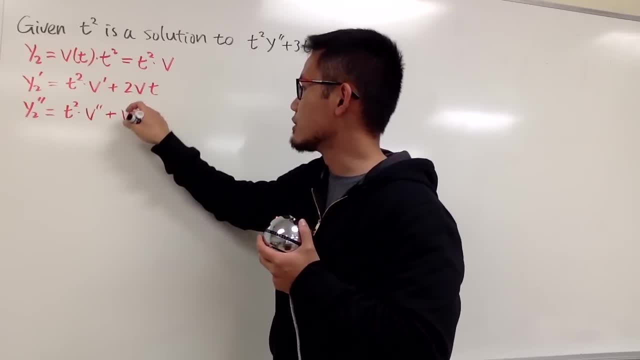 and then we add the second function, which is just phi prime, and then we multiply by the derivative of the first, which is 2t. So let me put down 2t like that, And now I will differentiate this. 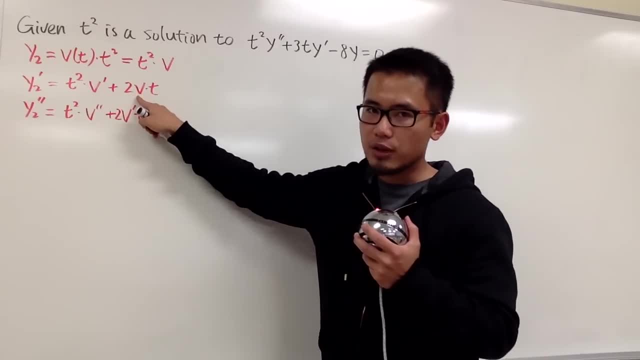 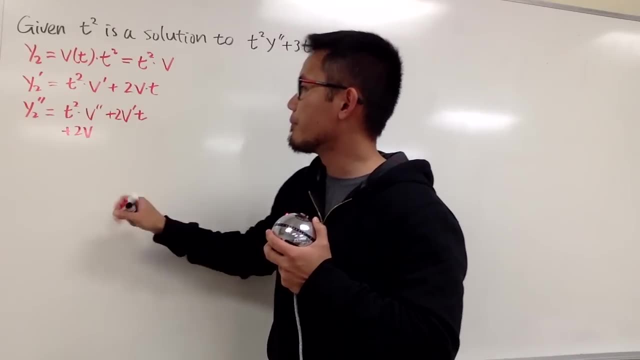 and of course, use the product rule. and I will look at 2phi as the first function, t as the second function, And let me put down 2phi first. right, We keep the first function, 2phi, and we multiply by: 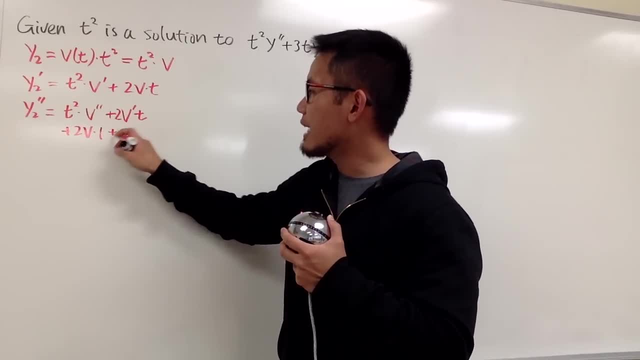 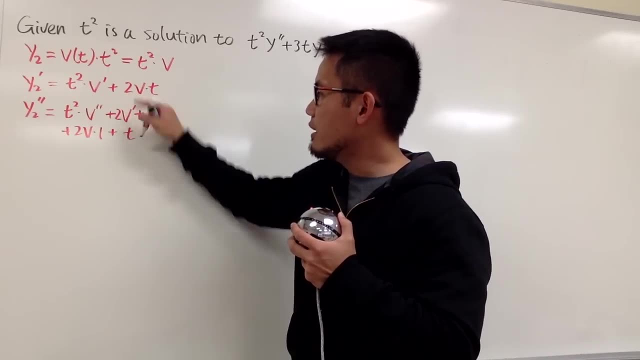 the derivative of the second, which is just 1.. And then we add the second function, which is t, And we multiply by the derivative of the first. Derivative of 2phi is just going to give us 2phi prime, like that. 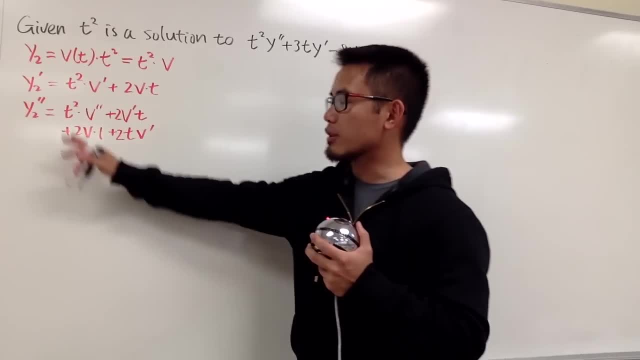 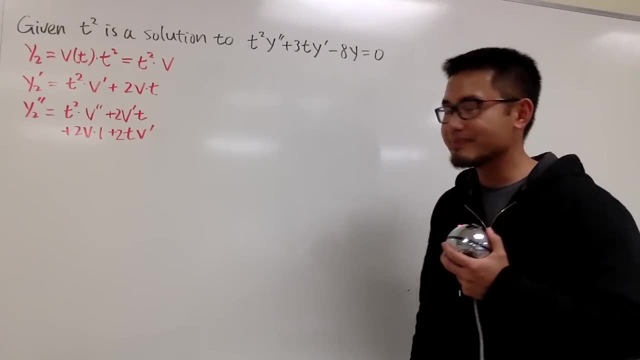 And now we have all the ingredients and we just have to plug in all this into this differential equation and then we'll try to solve for phi from there. So let me just put this down First. we have t squared. 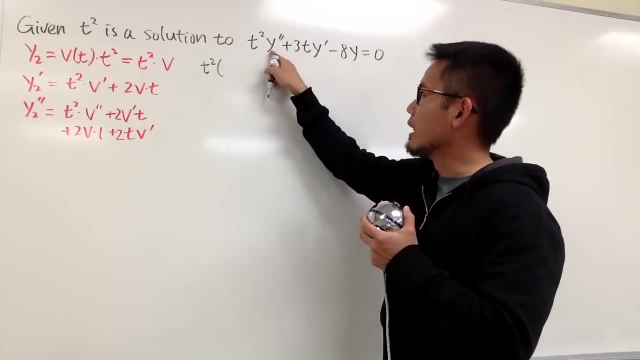 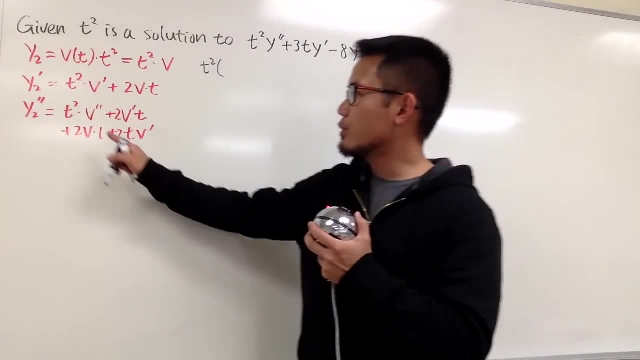 so let me write it down in the front and I will have to plug in y double prime, which is this expression here, and I am just going to put this down in order: phi double prime. that term goes first. okay, And I will put. 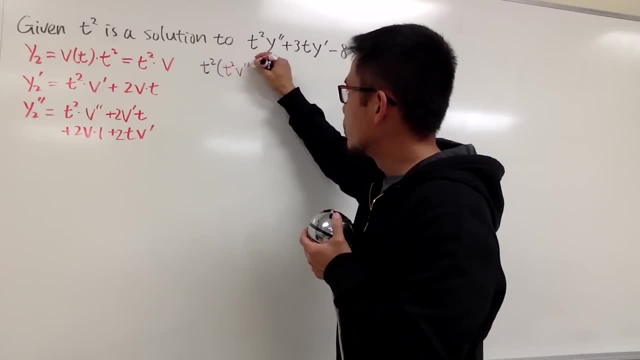 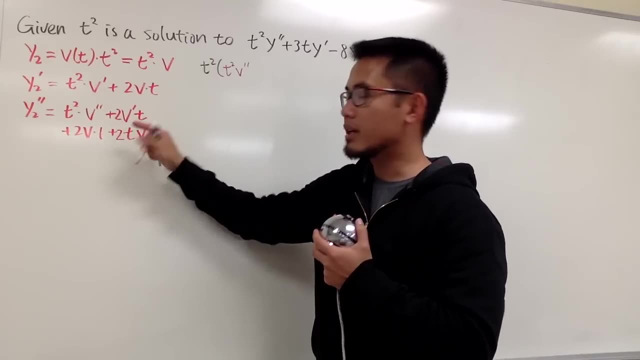 down the t squared phi double prime like this first, and I will look for the phi prime term, which is this and that, and both of them have phi prime t so I can combine the terms. So be sure to do so before you put it down, So you see that. 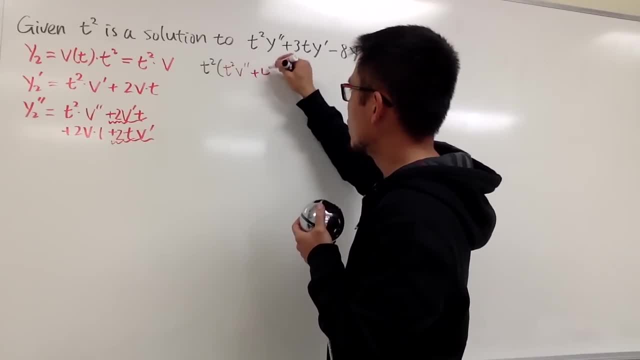 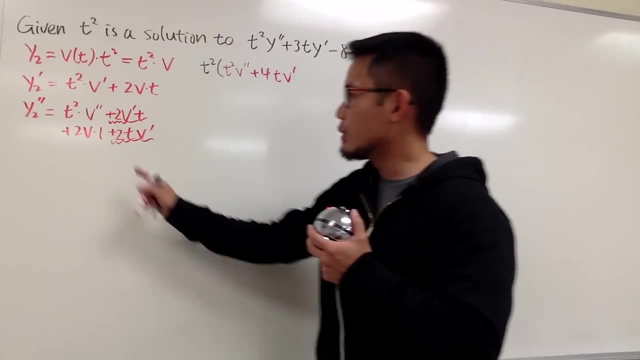 2, 2,, so of course plus 4, and let me put down the t first and then the phi prime, like that. And the last term that we have from the second derivative is just 2 phi times 1,, which is just. 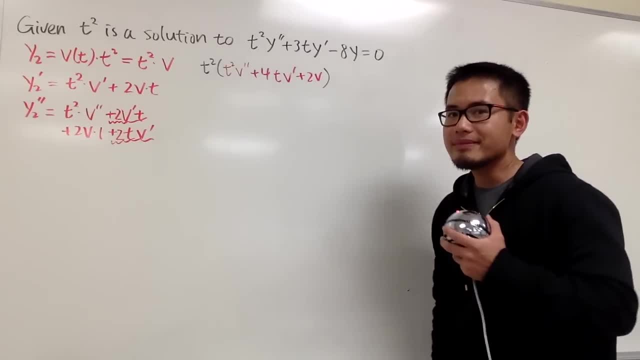 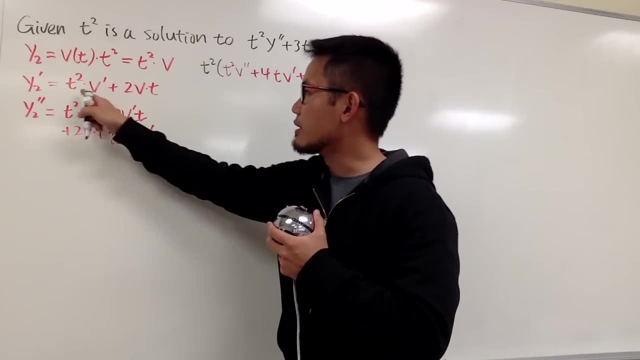 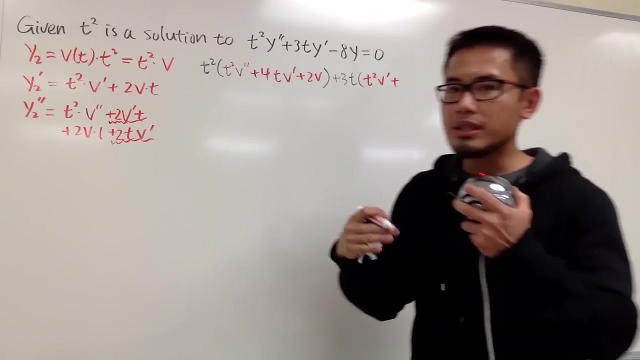 plus 2 phi, Okay, And next we have plus 3 t times y prime, which is just this. and let me put down t squared phi prime first, right here, and then we put down plus. and let me put down all the t's first. 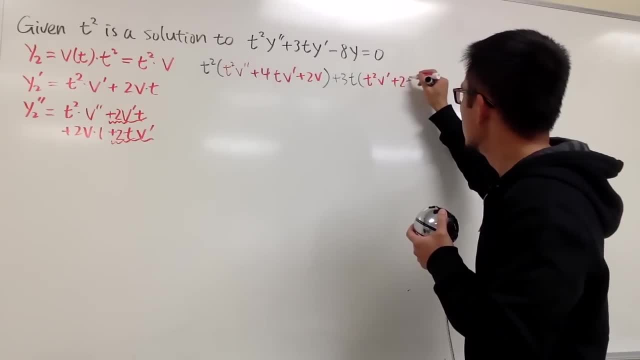 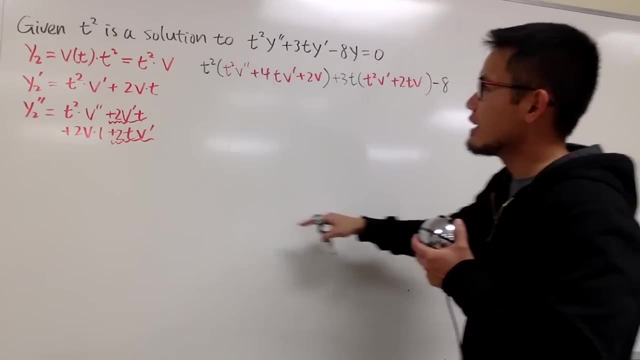 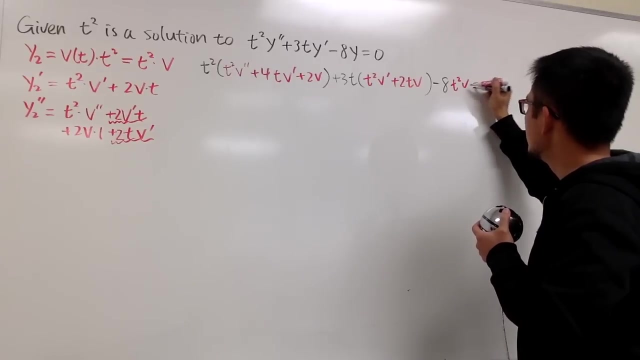 before phi. alright. So we have 2 t phi like that. At the end we minus 8, and the y is t squared times phi right. So we have 8 minus 8 t squared phi like that, and we still make this. 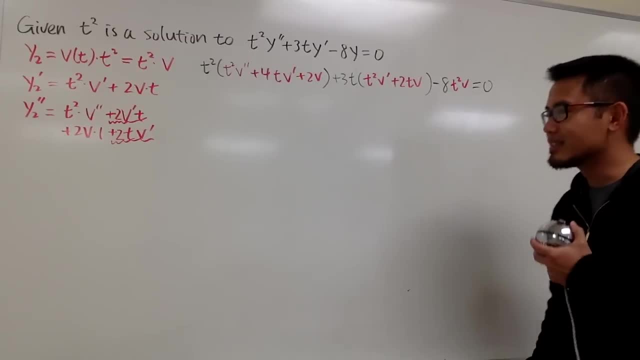 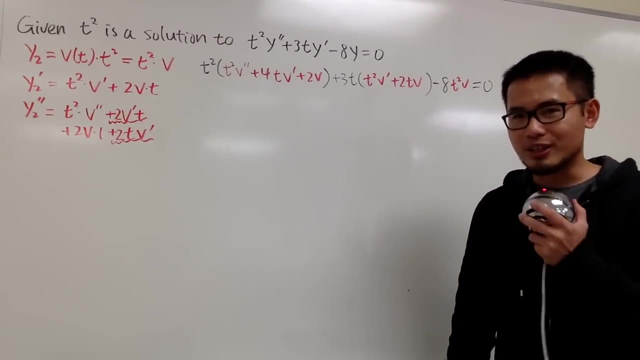 equal to 0.. And now let me just tell you guys something to look forward to. Whenever we're doing this right, the terms that was phi, the original phi, should cancel out, and you will see right, I don't promise. 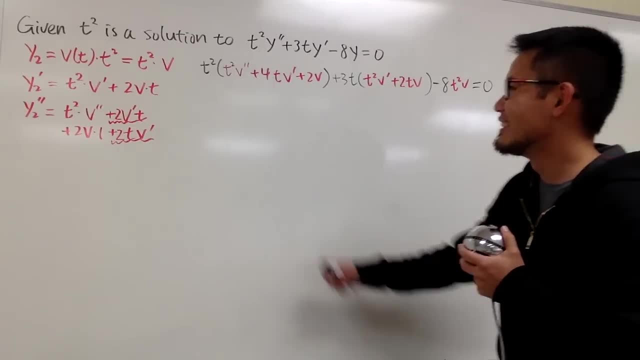 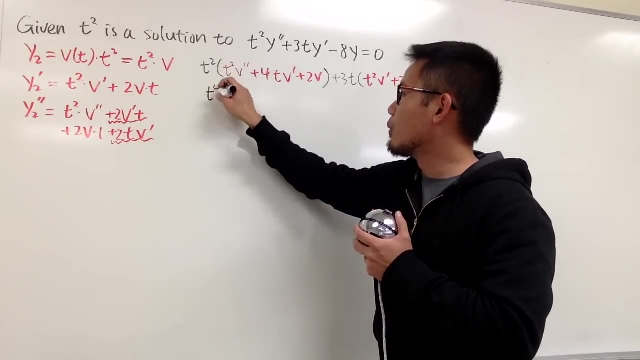 the other terms, but the term with phi should always cancel out. So now, let's see, I'm just going to distribute this t squared into this parenthesis, so we will have t to the fourth power, phi, double prime, and then we add it with: 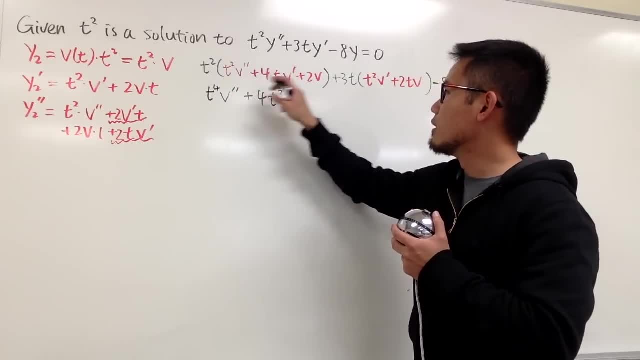 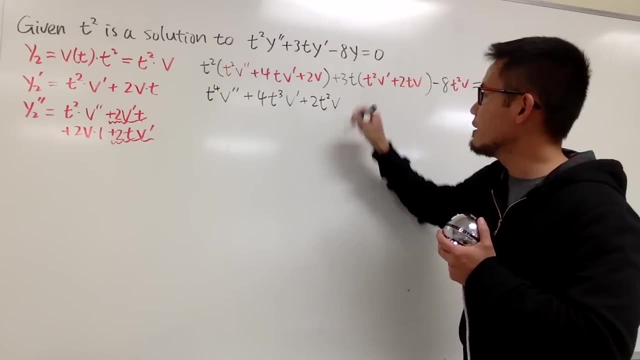 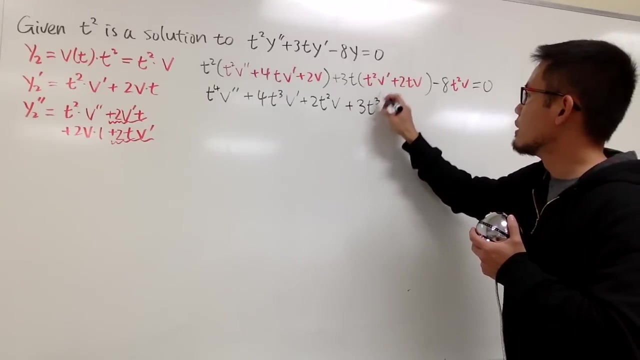 4 t to the third power phi prime, and then plus this times that which is plus 2 t, squared phi alright. And then we do this times that which is plus 3 t to the third power phi prime, and then we add it with: 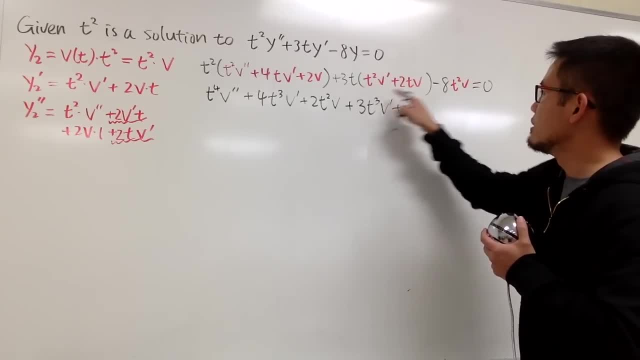 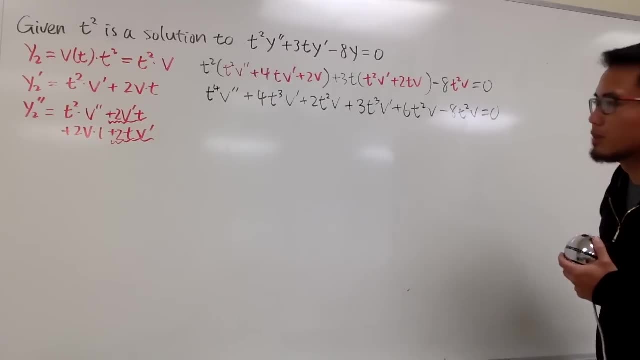 3 times 2 t, and so on, right: 3 t and then t squared, and then the phi. right here At the end we have the minus 8 t squared. phi still make it equal to 0.. Okay. 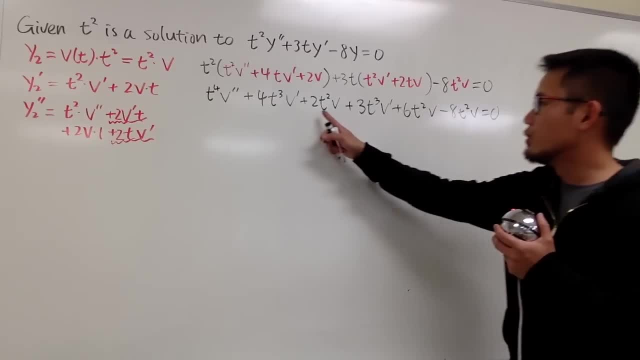 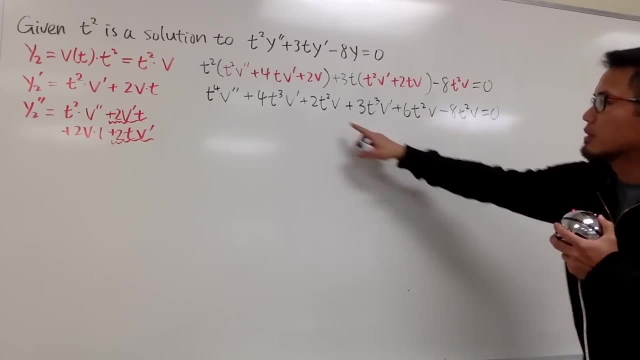 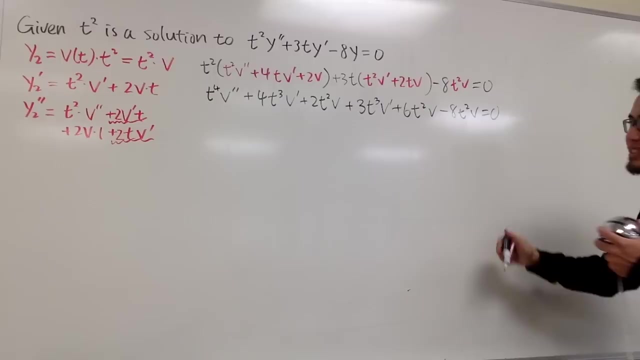 Let's see: Okay, we have the 2 t phi plus 6 t squared phi. right, 2 t squared phi, 6 t squared phi, that's 8 t squared phi, but we minus 8 t squared phi. so 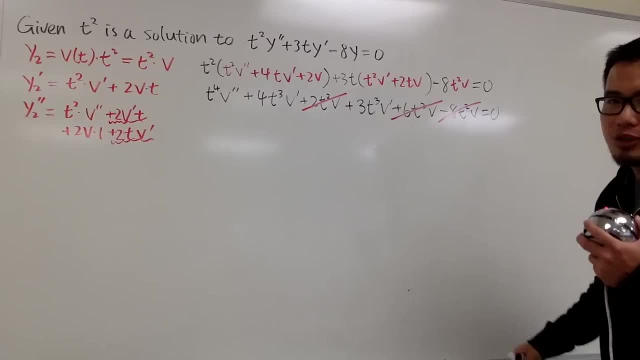 you see this, this that cancel each other. And you see all the terms have phi, they all will always cancel out. And now we see that this and that we can combine and this is pretty much stays the same, right, So in. 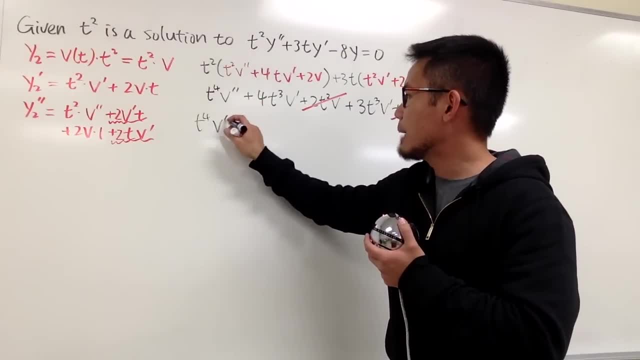 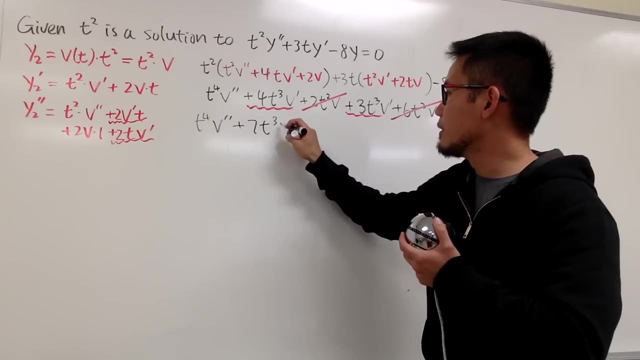 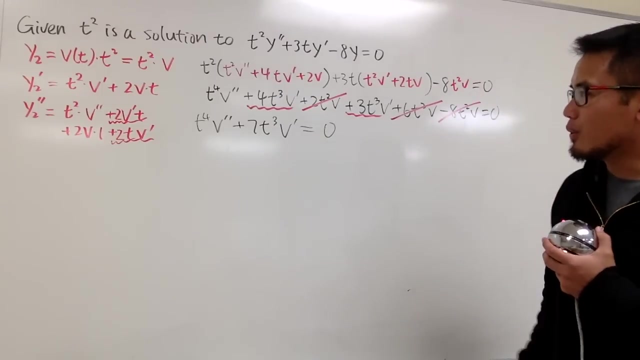 other words, we have t to the fourth power phi double prime and this and that together- let me just indicate that we are combining terms- It's plus 7 t cubed phi prime, and this is equal to 0.. Okay, so from. 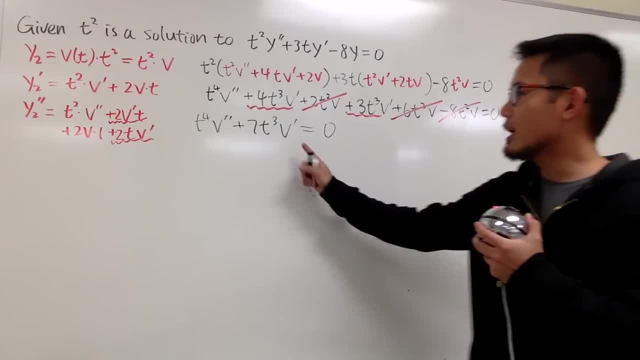 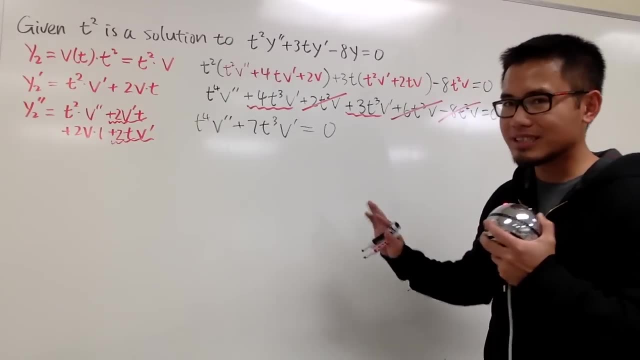 here can we solve for phi? Well, we see that we have the first derivative only and the second derivative right here. right, We don't have the original, So we can do some substitution, right? So in terms of this, right here, we just have the derivatives only. 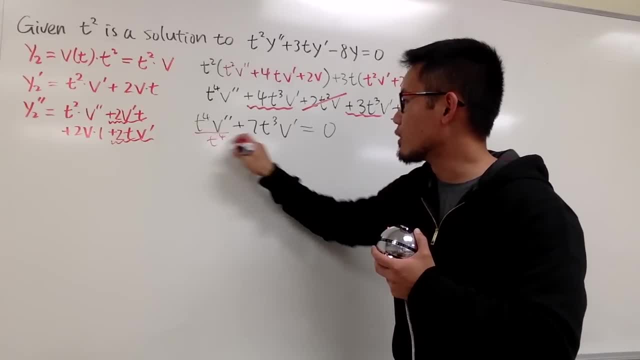 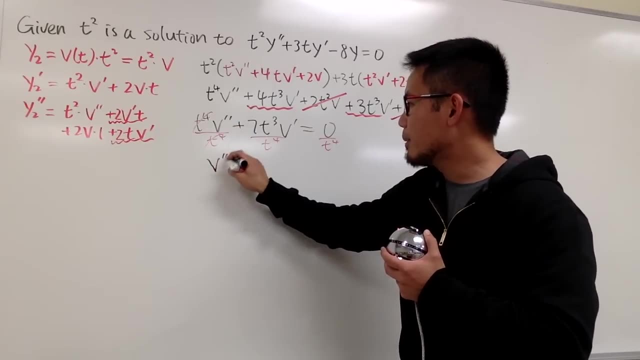 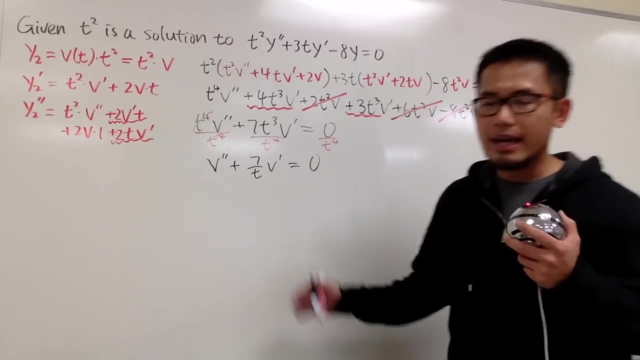 And what we can do is, of course, let's just divide everything by t to the fourth power, and in another word, we will look at this as phi double prime plus 7 over t, phi prime is equal to 0, and from here this: 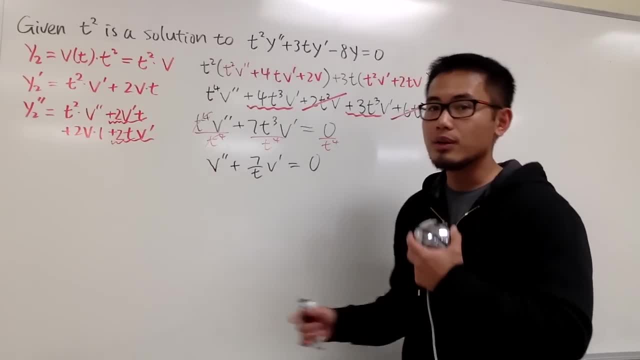 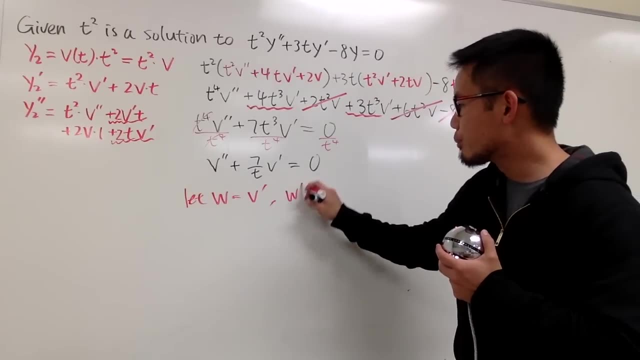 is the first derivative. This is the derivative of the first derivative. We do some substitution. we let w equals to phi prime. In another word, w prime will be phi double prime, right. So we can look at this right here as w. 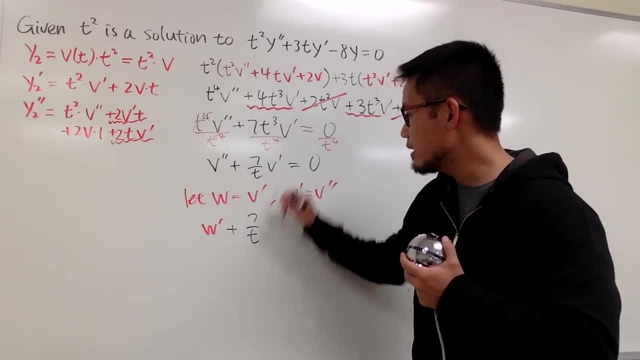 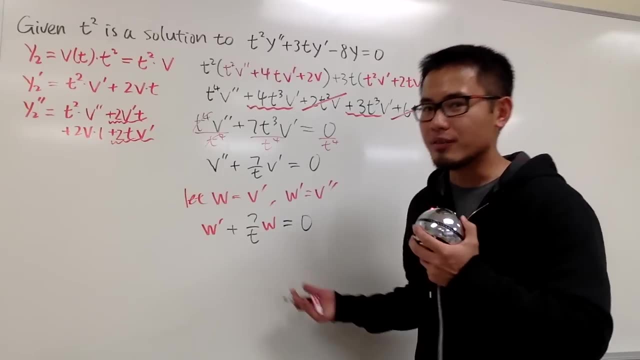 prime plus 7 over t, This is just the regular w, and then this is equal to 0.. And I can just solve this by separating the variables and I'll show you. Let's move this to the other side and allow me to write down w prime. 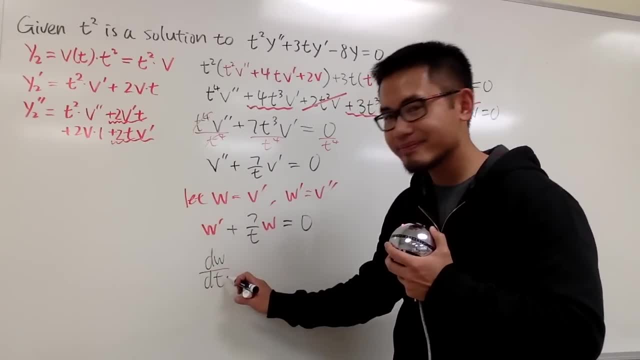 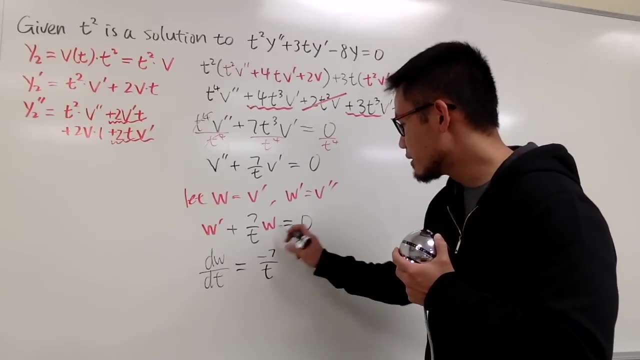 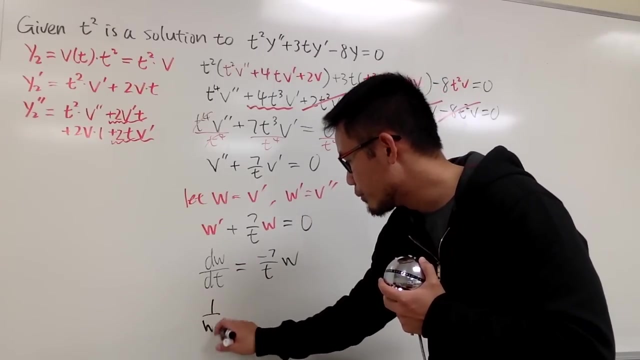 as dw dt right, I'll move this to the right-hand side. so this is equal to negative 7 over t w like this, And now I will divide w on both sides, so I will get 1 over w here. 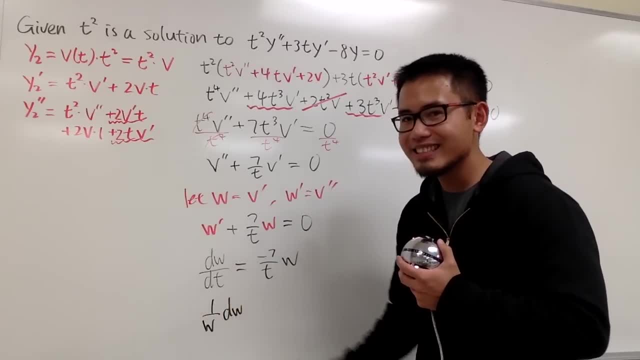 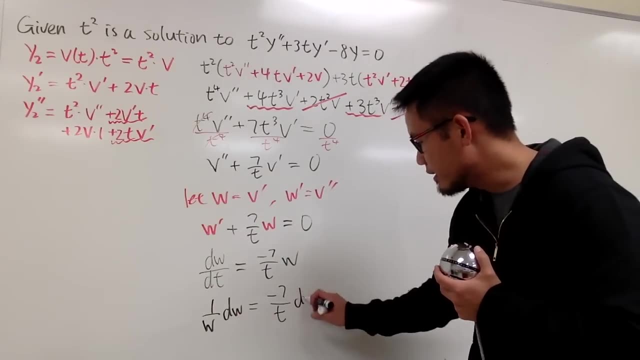 and I will keep the dw on the left-hand side and this is equal to negative 7 over t and I will multiply dt on both sides. So we have this right here And now we can separate. we separated the variables and now we can just go ahead. 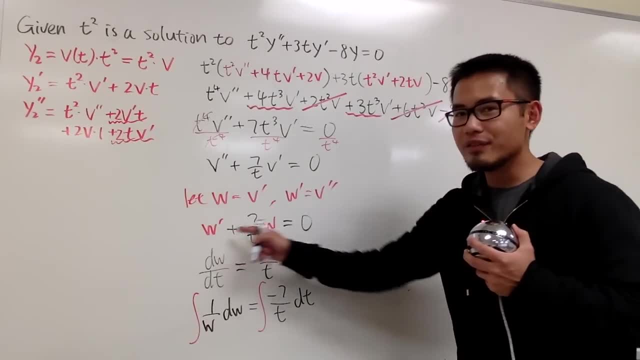 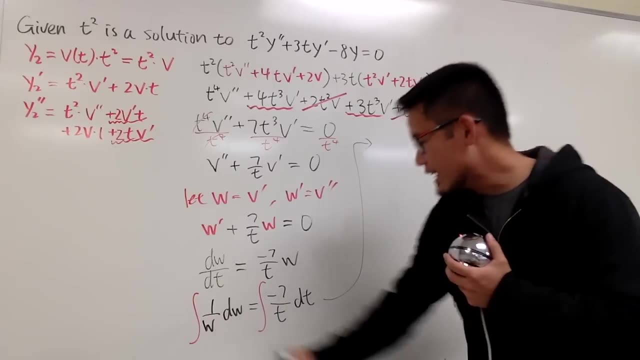 and integrate, integrate, And of course, if you want to just solve this by the integrating factor, you can do the same as well, doesn't matter. Um, on the left-hand side we get ln absolute value of w, and on the right-hand side we get equal to. 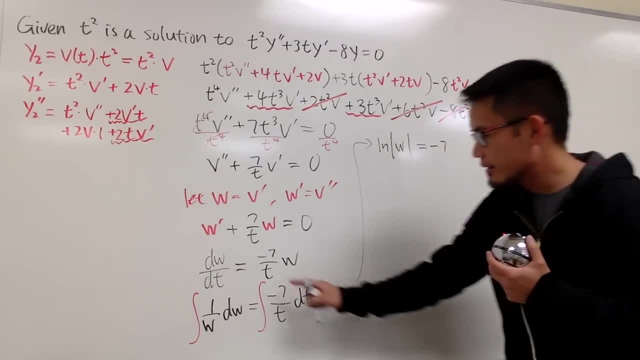 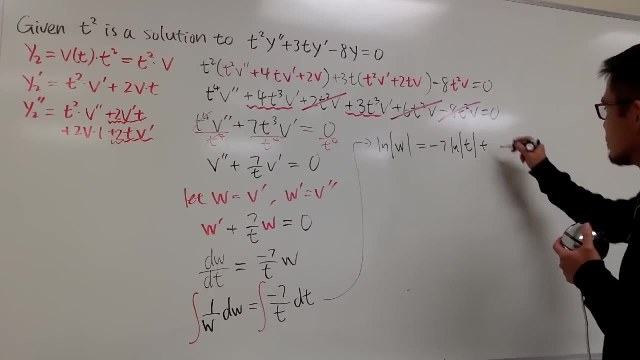 put down the constant, which is negative 7, and the integral of 1 over t. dt is ln, absolute value of t. and here we put down a constant right, And let me just put down plus k1 right here. Alright, I want to solve for. 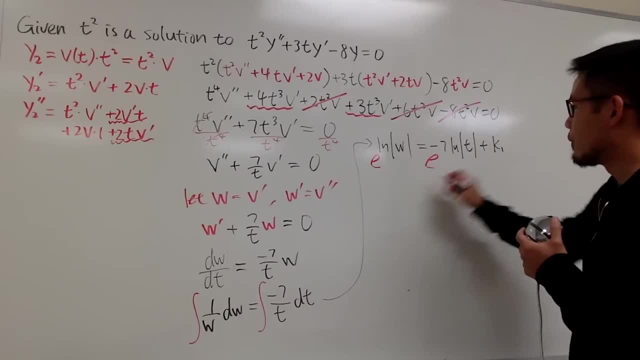 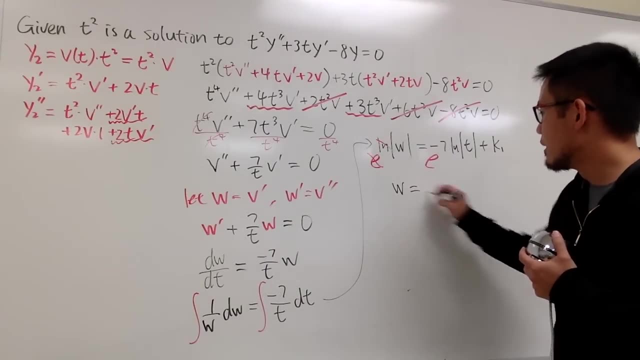 w from here. so let me just do e to this power and e to that power. this and that will cancel, and you know the deal. The absolute value doesn't matter. Let me just write it down as w here, And then you also know the deal. 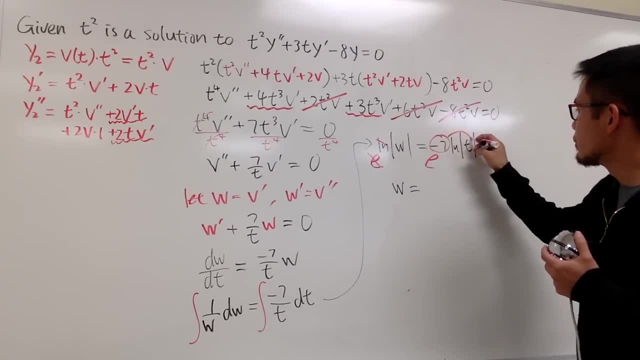 Right, here you are going to bring the negative 7 to the power here, right? So let me just write this down as: e to the ln absolute value, t to the negative 7 here, and you know we have to multiply by. 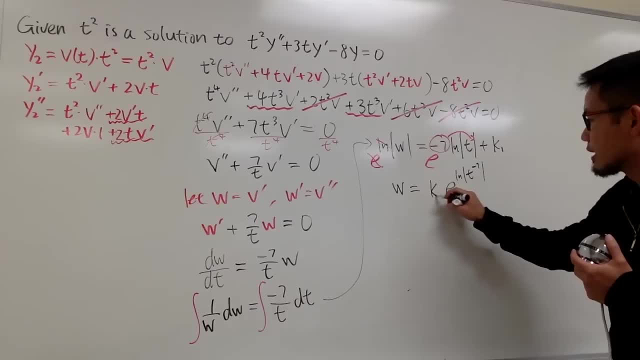 e to the k1,, which is the same as another constant. so let me put down k2, like this: And you know the deal, this and that will cancel. and you know the deal, the absolute value doesn't matter. In another word, w is equal. 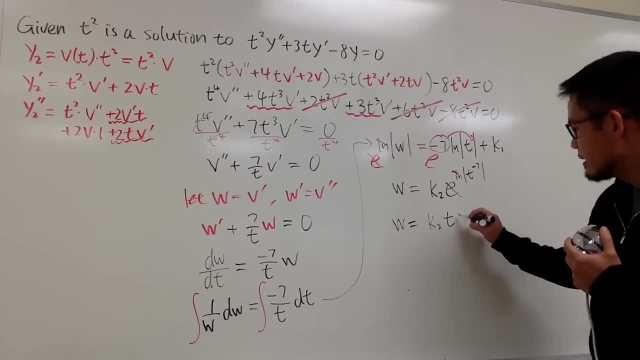 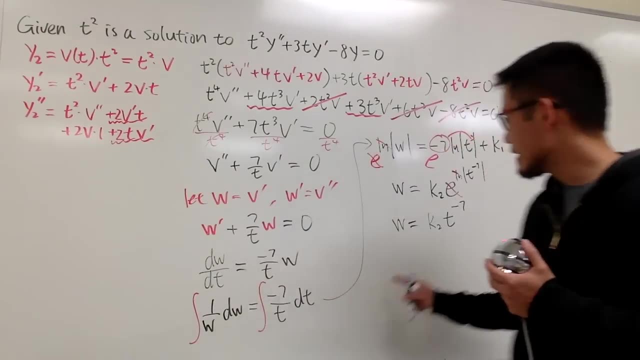 to k2 times t to the negative 7.. Alright, what's w? w is the same as v prime, and I can just write this down right. So we have: v prime is equal to k2, t to the negative 7.. 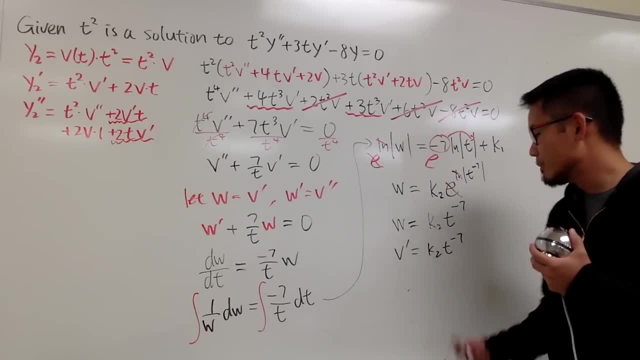 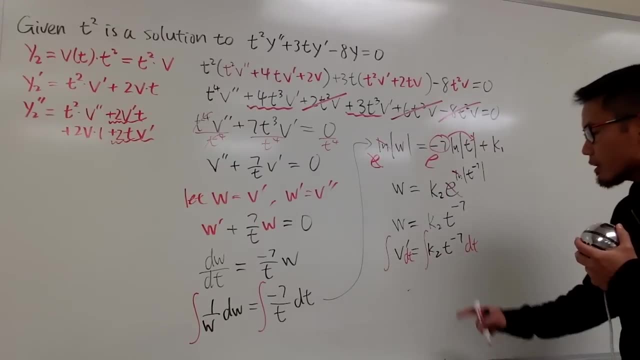 If you want, you can write this down as dv, dt, but it doesn't really matter that much, right? We can just go ahead and integrate. integrate respect to with respect to dt though. So on the left hand side, we see that we just have v by itself. 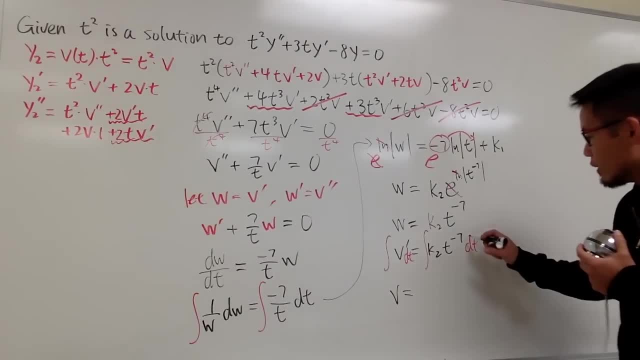 and on the right hand side. what do we do with this? Well, this is a power right t to the negative 7, so I will add a 1 to it. negative 7 plus 1 is negative 6,. 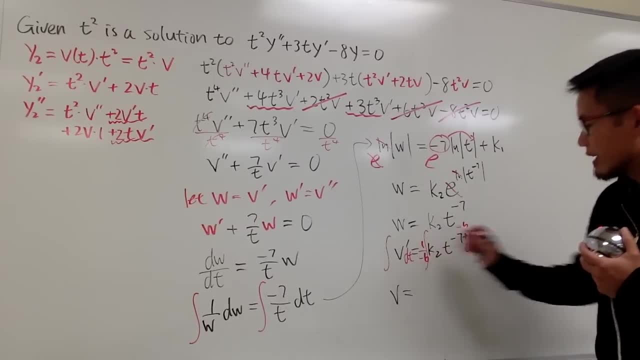 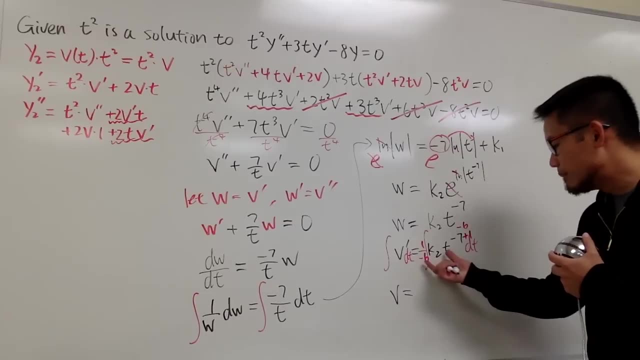 and then I will divide it by negative 6, which is 1 over negative 6, like that, right, Okay, k2 is a constant. Multiplying by 1 over negative 6 is another constant. so let me just put this down as: 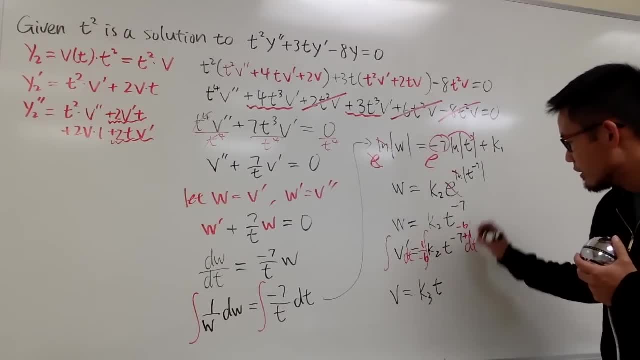 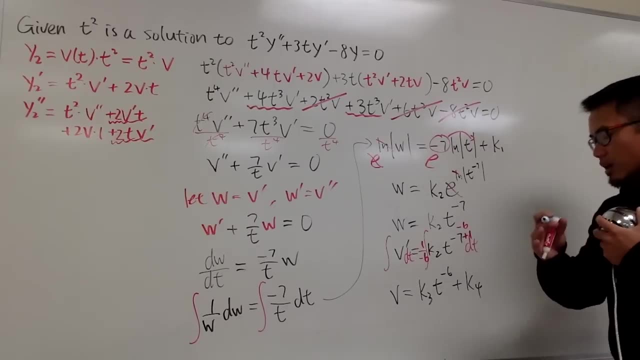 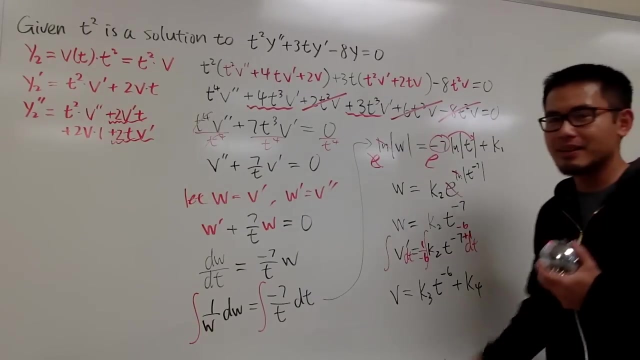 k3, and this is t to the negative 6 power. and technically, right here, I still have to add another constant, so I will put down k4.. Okay, this is how the v will look like. alright, And now we are pretty much done. 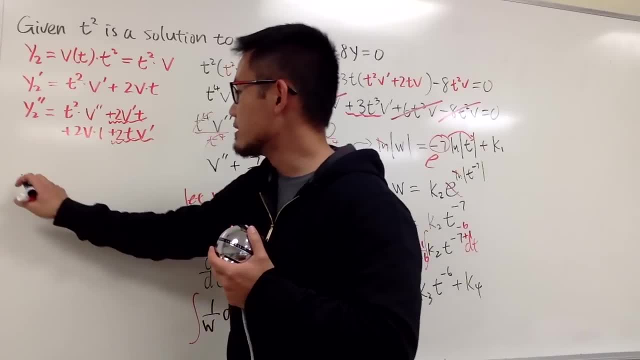 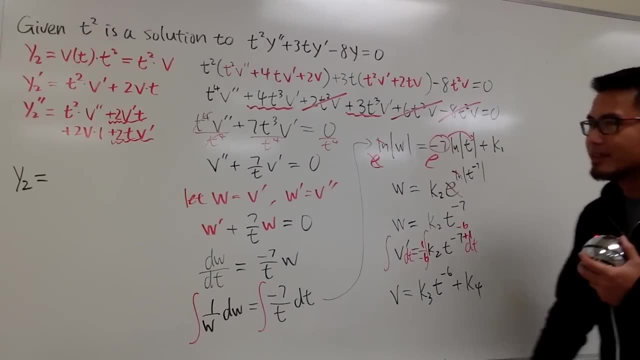 I will come back to here for you guys, Because now I can say y2,, which is going to be v of t, and we found it. It's right here. It's right here, isn't it? So let me just write this down. 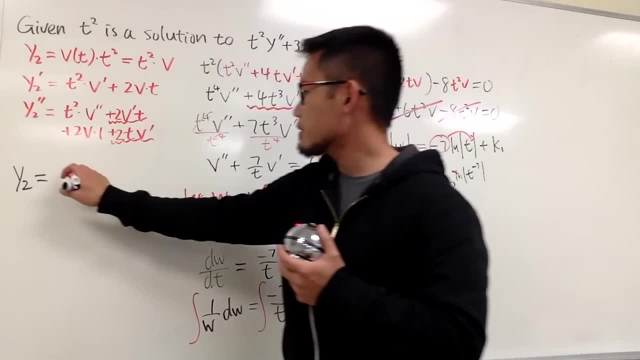 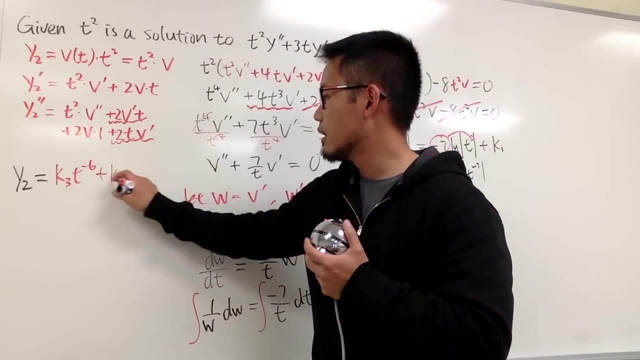 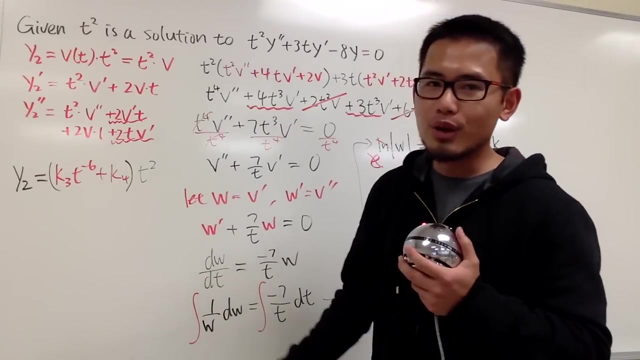 It's going to be k3, t to the negative 6, and we add it with k4, right, We take this and we multiply by t2, right? Okay, of course we can just multiply, multiply, so you see. 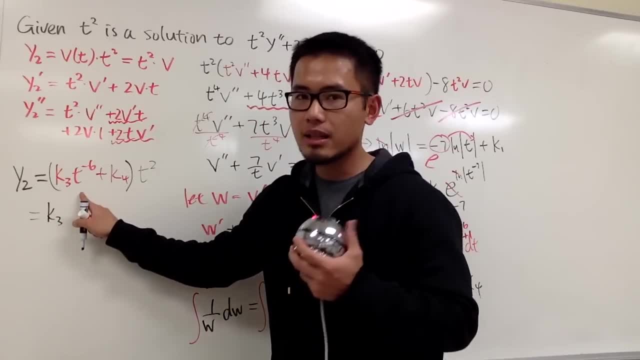 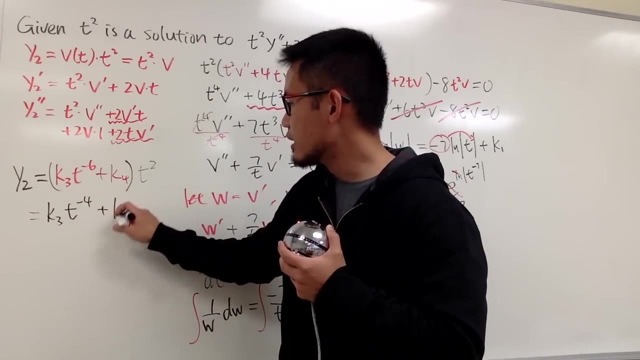 this is going to give us k3. this times that the power. now it will be to the negative 4.. k3 t to the negative 4, and then we add it with k4- t2.. Okay, so this is how. 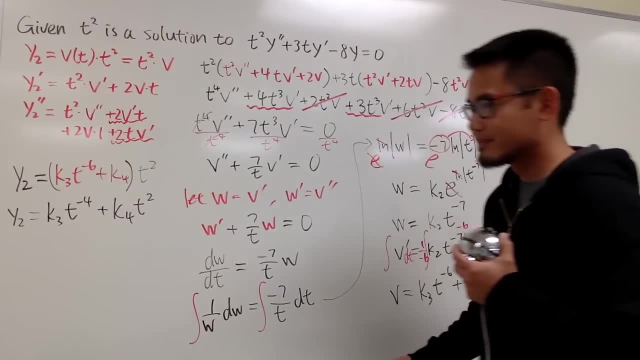 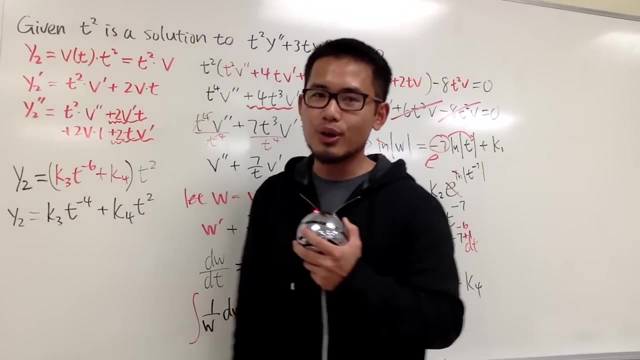 y2 will look like, based on all the computations that we just did. Okay, what's the new guy? This right here? it's given, isn't it? It's just a constant multiple of the original, so it's not new. 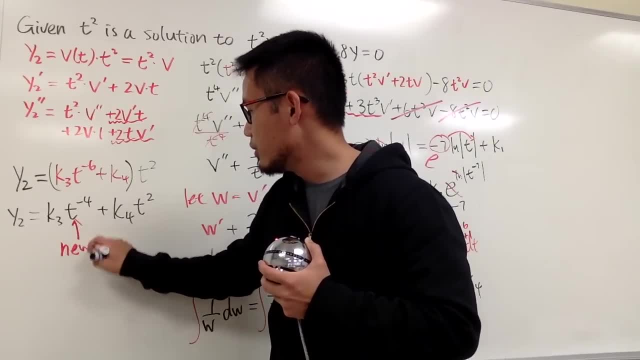 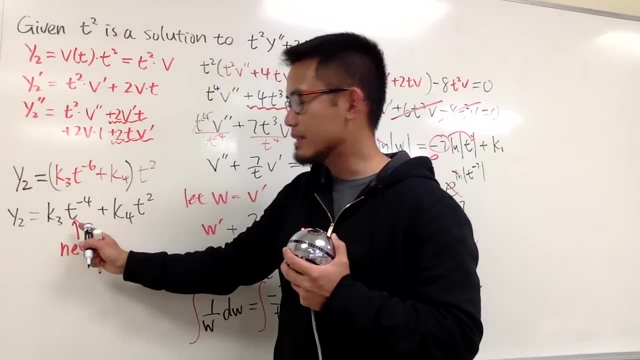 The only thing that's new is this: This is the new building block for the solution. So, altogether, you know, this is the first building block, this is now the second building block and we just include the constant multiples and that will be the answer. 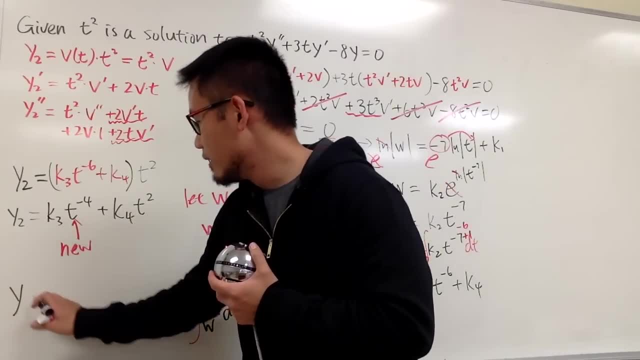 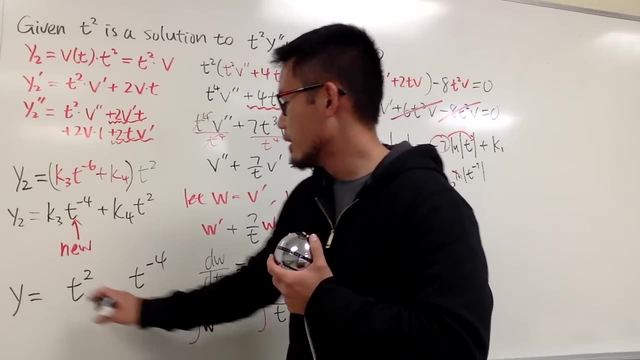 So I'll just write down all the answers right here together: y is equal to the first building block, which is t2,, and the second building block is that t to the negative 4 constant multiples of c1,, c2, and then 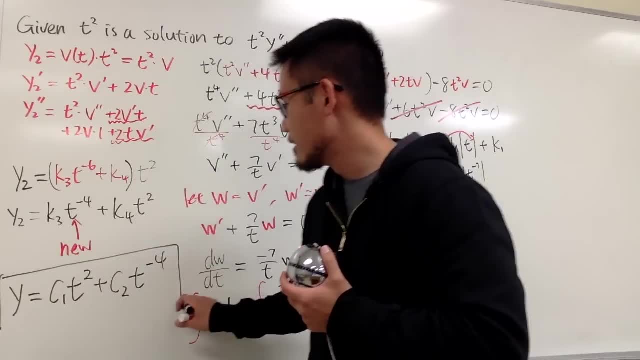 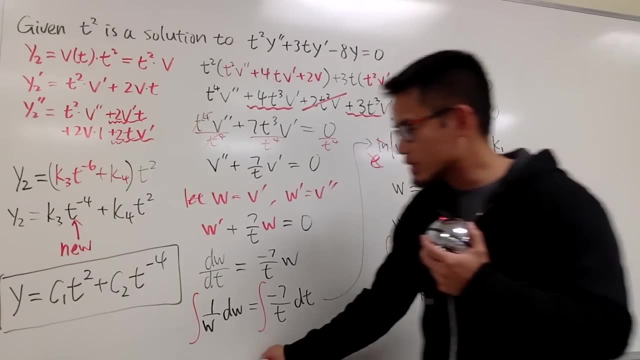 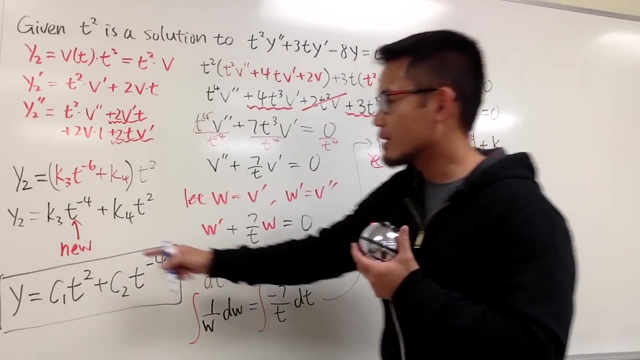 we add them together. That's it. This is the overall answer, the general solution for this differential equation. And just for fun, before we go, I will show you. this is in fact the solution to that as well, And I'm not going to put. 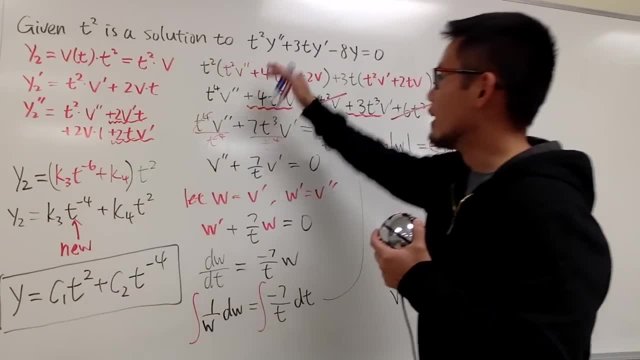 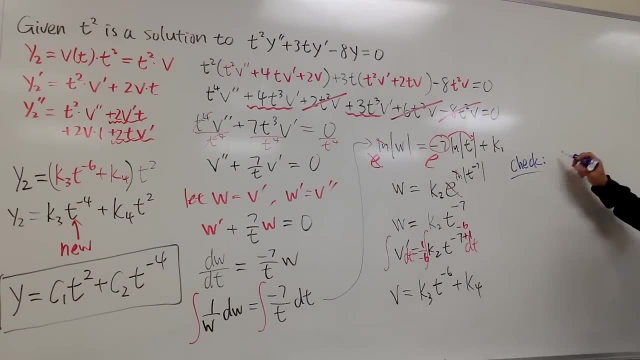 down the constant multiple, because if you have the constant multiple, you still have that constant multiple anyway. So just a real quick check right here. alright, This is just to check. So if y is equal to t, to the negative 4, and then I will. 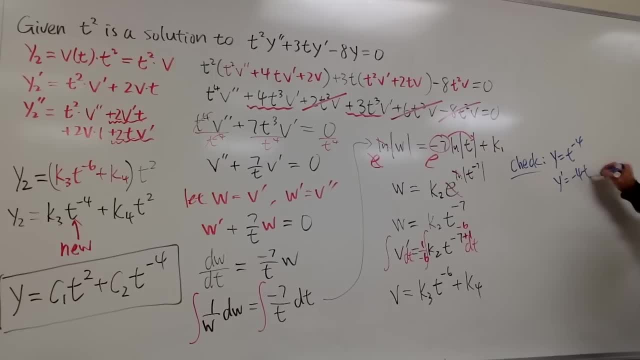 just differentiate this. we see y prime is going to be negative 4,, t to the negative 5, and then one more time: y double prime is going to be positive 20,, t to the negative 6.. And now we just have to plug in all this. 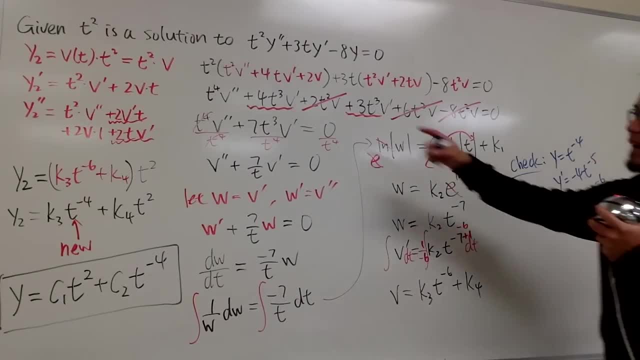 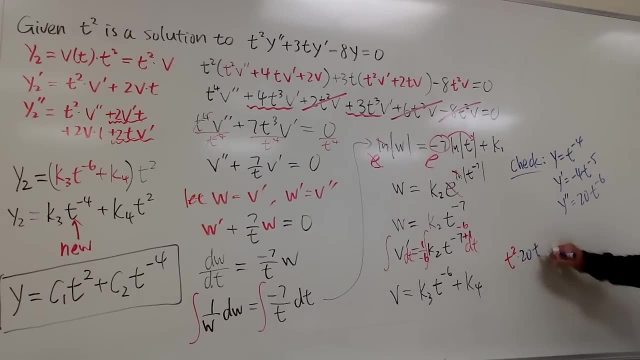 into the differential equation and you will see we will have first t squared times y, double prime, right? So let me write it down: t squared times that, which is 20, t to the negative 6.. And then we add it with: 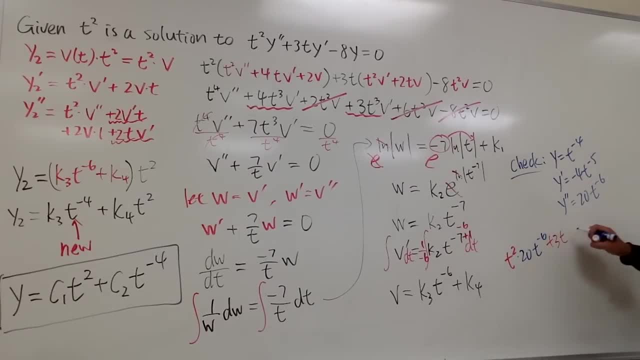 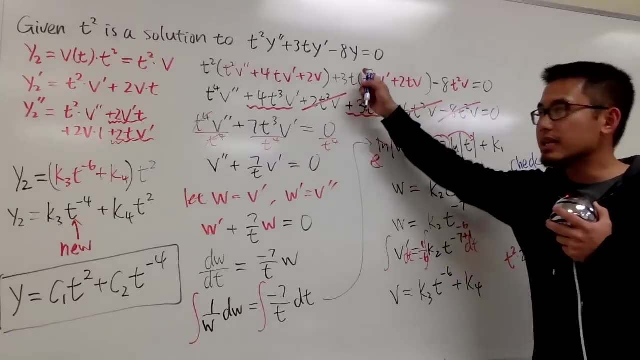 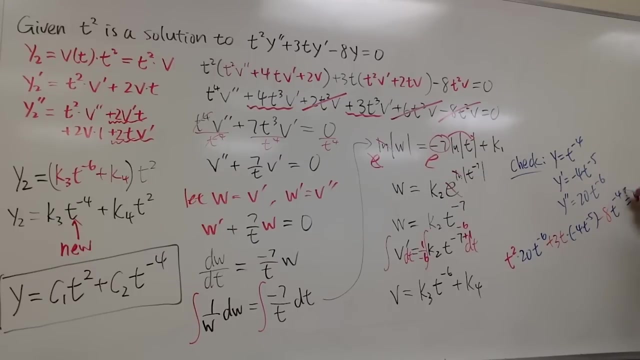 3t, and the y prime is that which is multiplied by negative 4, t to the negative 5.. And then at the end we minus 8.. Why is that? Because t to the negative 4.. Do we get 0?? 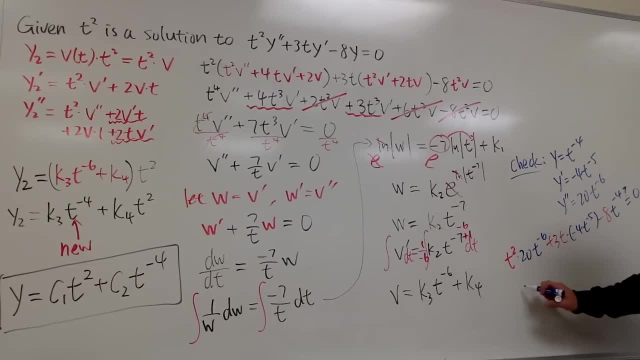 This is the question mark. Do we get 0?? Well, here is 20,. together, the power is going to be negative 4.. This and that is minus 12, and once again, the power is also negative 4.. And this right here is. 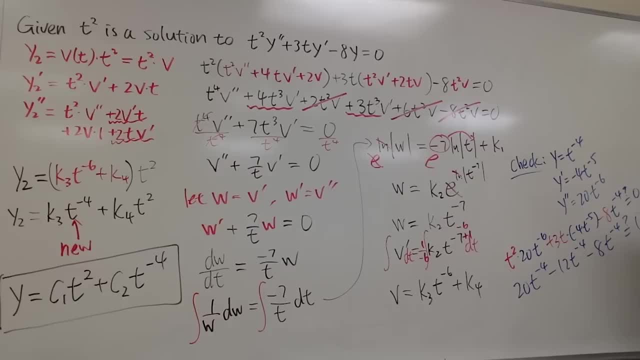 minus 8, t to the negative 4.. Does this give us 0?? 20 minus 12 is 8.. Minus 8 is 0.. Right, They are like terms and 0 is of course 0..